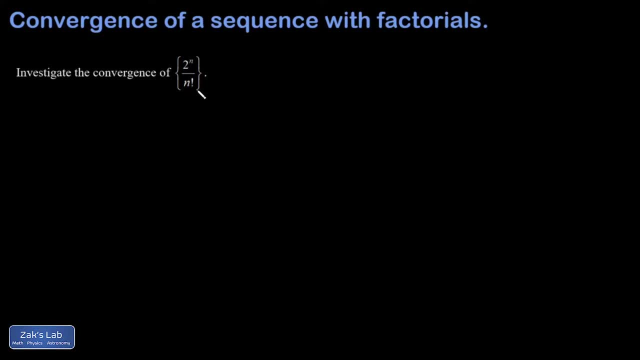 So, undoubtedly, the numerator and the denominator are both getting very large as n goes to infinity. Factorials and exponentials both grow incredibly fast and in a sense I'm just asking which one of them wins here. So let's look at a1, plug in: n equals 1.. 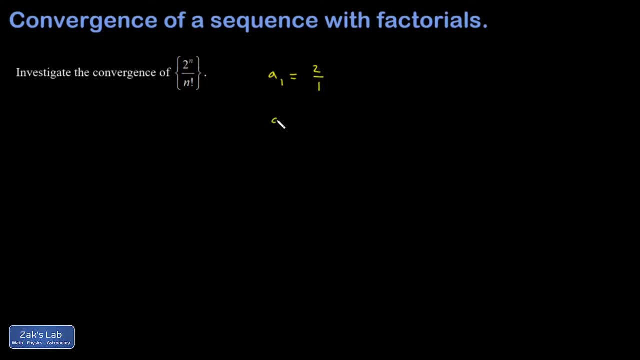 And I get 2 over 1 factorial, which is 1.. Now let's look at a2.. In the numerator, I have 2 squared, which is 2 times 2.. In the denominator, I have 2 factorial, which is 2 times 1.. 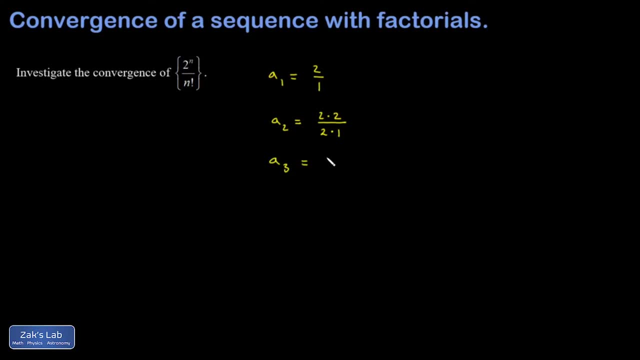 Let's look at a3.. It's going to take a while to see what to do here. In the numerator I have 2 times 2 times 2.. And in the denominator I have 3 times 2 times 1.. 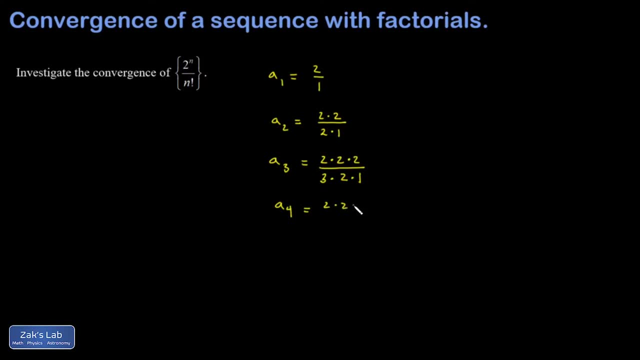 a4. In the numerator I have 2 times 2 times 2 times 2.. And in the denominator I've got 4 times 3 times 2 times 1.. So you might be getting a sense at this point that the factorial is winning. 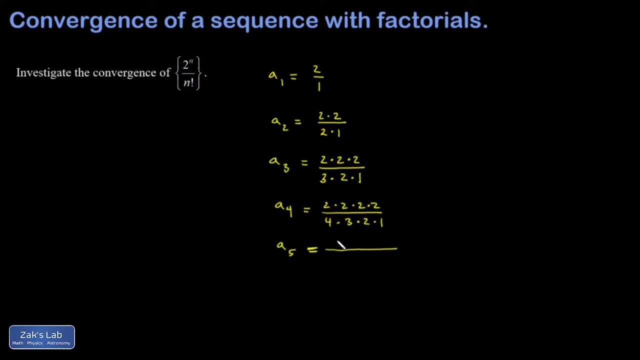 because it's tacking on a term that's bigger than the corresponding term tacked on in the numerator every single time. All right, and now it's time to sort of cleverly set up an inequality here. What I notice in a2, so n, is 2 here. 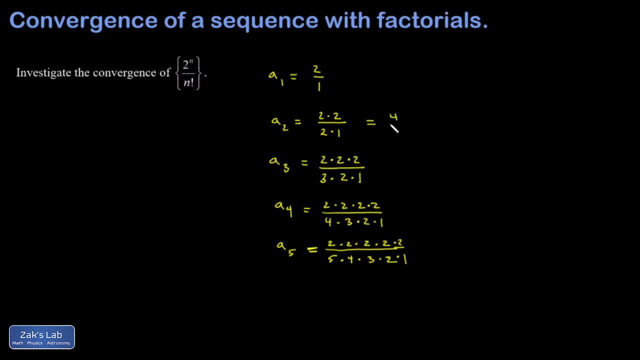 I could say that a2 is equal to 4, because I have these two factors in the numerator over n. Now it might seem a little curious that I would write it that way, but let's try to do something similar in the next example. 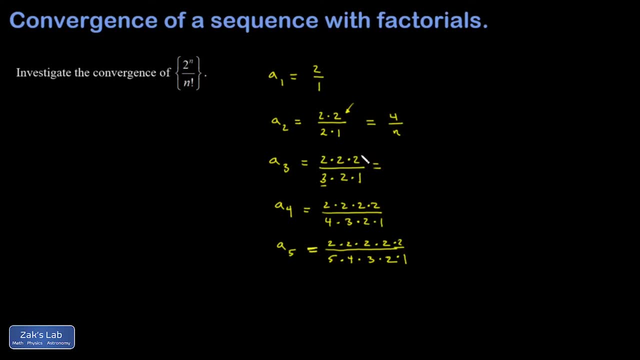 So n is 3.. And if I cancel one of these factors of 2, I end up with again 4 over n. So now let's look at a4. And I'm not going to have an equality anymore. I'm going to end up with an inequality. 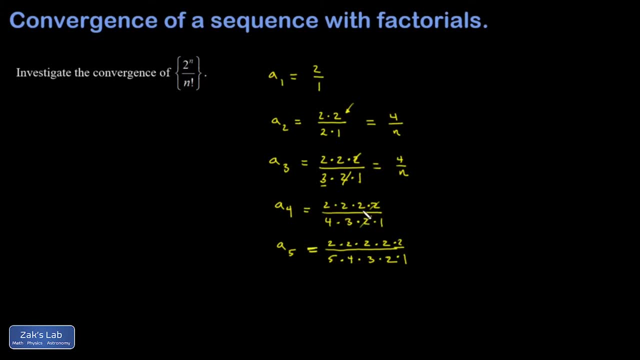 So I'm looking at sort of pairing up. I can cancel these 2s, But I can't cancel another 2.. But I do see that I have a 2 thirds that I could highlight, And so what I'm going to say is: 2 thirds is less than 1.. 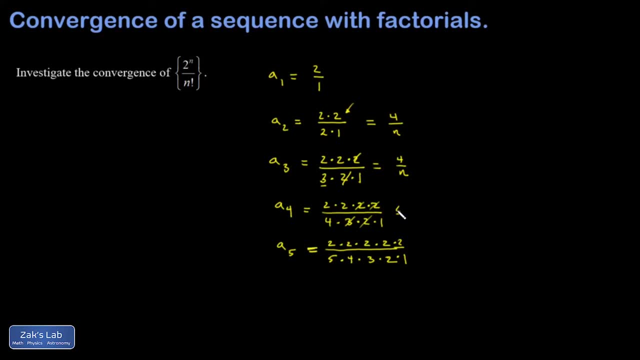 And so this expression on the left is going to be less than, And I'll go ahead and throw in an or equal to to cover those first two cases. And I have a 4 in the numerator And then I have An n in the denominator.